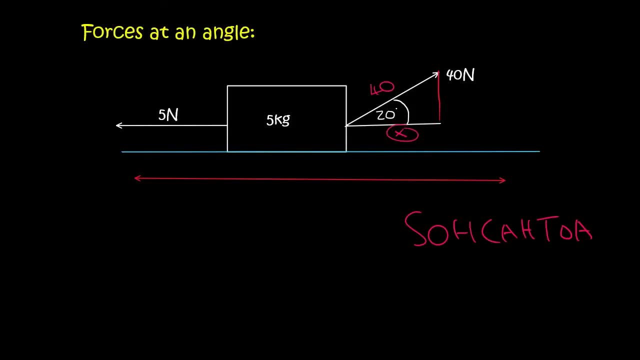 already have the 40,, which is your hypotenuse. You're looking for the adjacent, and so that's cos. So what we can do is we can say: cos 20 is equal to the adjacent over the hypotenuse, which is 40, and so x is equal to 40 cos 20,, which is 37.. 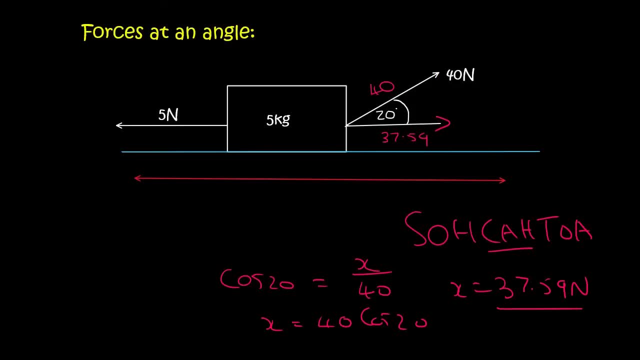 And so now we can comfortably or confidently say that this object is going to go to the right, because that 40 newtons, when you break it into its horizontal component, it's 37.59.. And so then, if we wanted to work out the acceleration of this object, we would use Fnet, equals to ma, But when? 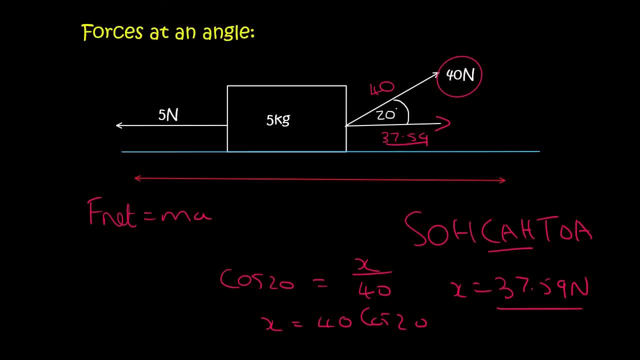 you'd write this equation, it's either going to be to the right or to the left as positive, so you must tell the teacher what you're choosing as positive. So the equation is either going to be to the right or to the left as positive, so you must tell the teacher what you're choosing as positive. so the 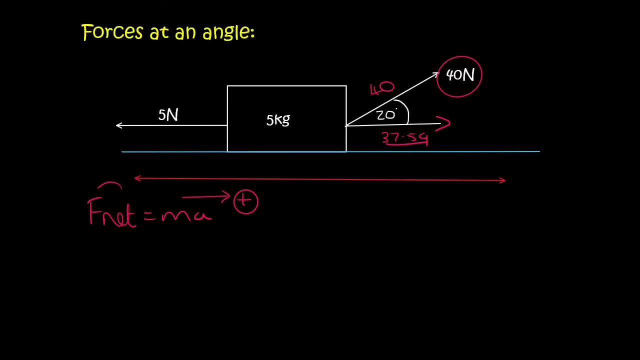 easiest one would be to choose the right as positive. And so, Fnet, remember that's like your business profit. So, to the right, you've got 37.59.. To the left, you've got 5.. You do not use the 40,. 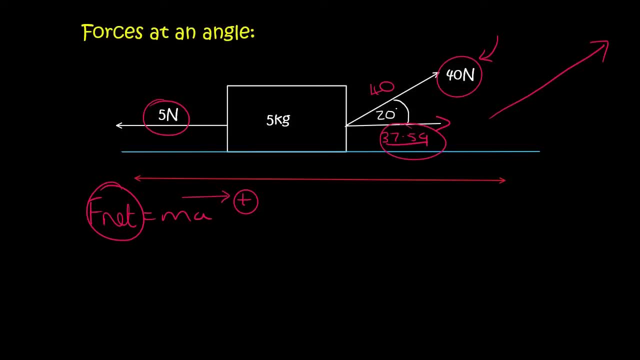 because the 40 is some random direction. You only, in a question like this, you only want to work in the horizontal direction. Kevin, what about the vertical direction? Excellent question. Not a lot of people ask me that I have made this 5 kilogram object heavy enough so that it won't be able to. 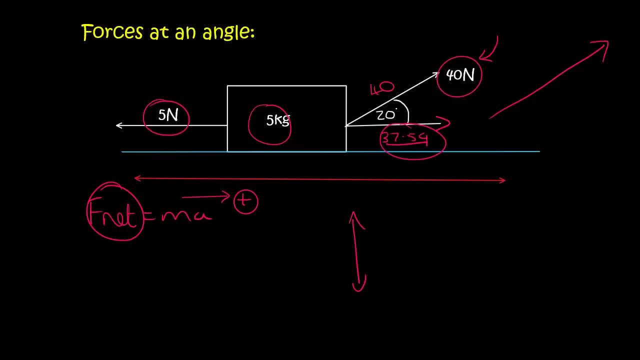 lift. Let me prove that to you, because I don't want to lift it, I want to lift it, I want to lift it. I see so many teachers getting this wrong in exams where they actually make the object so light that technically the question doesn't work out. But most teachers they miss that. So if we're 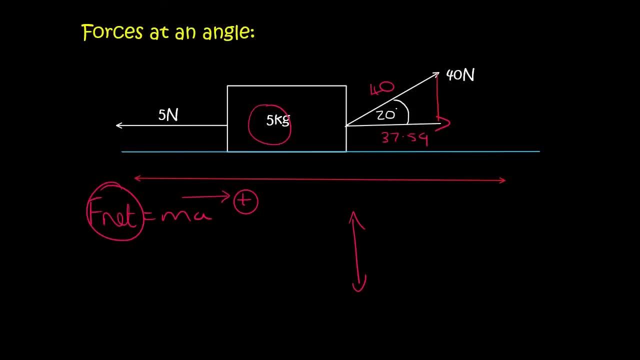 to construct our little triangle again, and you'll never have to do this in an exam. I just like to check up on teachers. So if we look at the opposite, and we already have the hypotenuse, well, that's sin. So we can say sin 20 is equal to the opposite, which I'll call y. 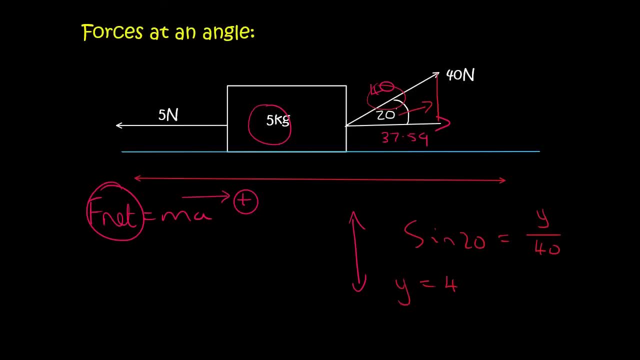 over the hypotenuse, which is 40. And so y is equal to 40 times by the sin of 20.. And so that's 13.68 newtons, And that's going up. Okay, so that's 13.68 newtons. 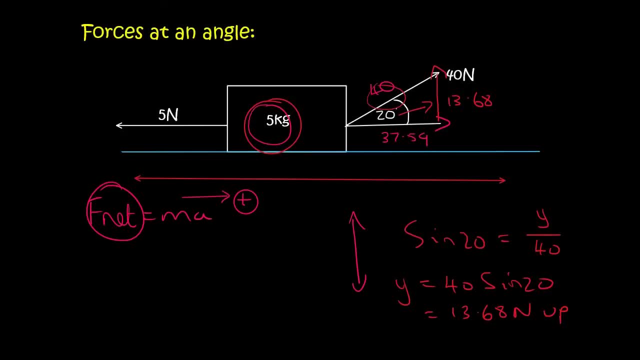 up. Now we need to look at this object. Well, the mass of this object is 5. And so its gravity is 5 times by 9.8, which is 49 newtons. So the gravity is 49 newtons down the upwards force. 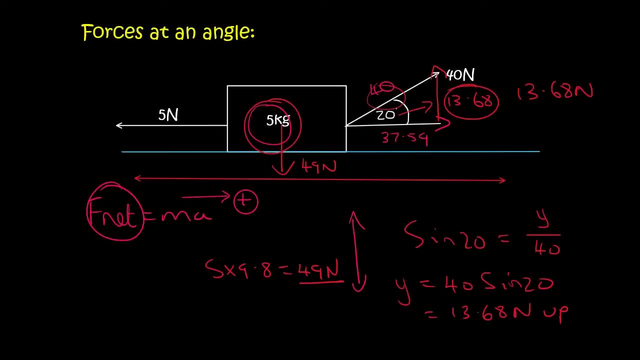 is 13.68 newtons, And so that upwards force is not going to be enough to lift the object off the ground. But then, Kevin, why is the object not going through the floor? Because that's 49. And that's 13.68.. That's not balanced. Aha, that's where the normal force comes in, guys. So the normal force. 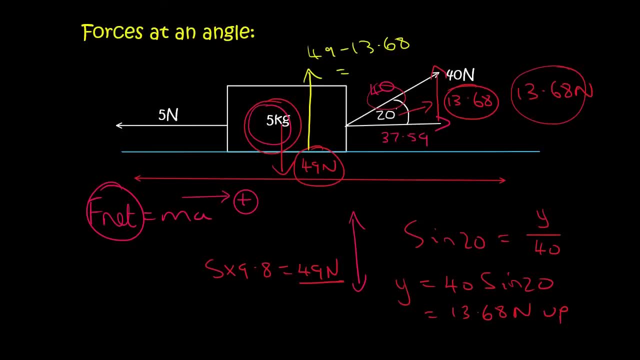 would be 49 minus 13.68. And that's 35.32 newtons. And so all the upwards forces, which is your normal force, and the this 40 newtons in the upwards direction, those two together add up to: 49.. And so the total upwards force is going to be 49 minus 13.68.. And so the total upwards force is going to be 49 minus 13.68.. And so the total downwards force is going to be 49 minus 13.68.. And so: 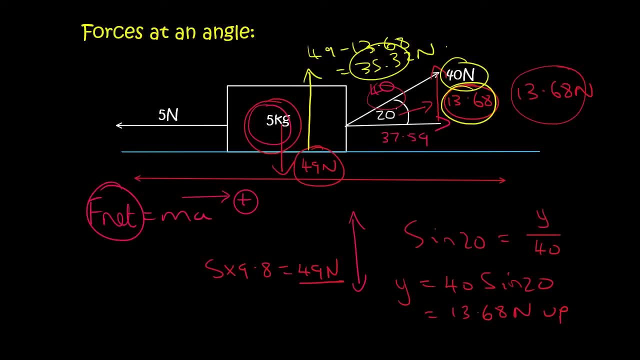 the total downwards forces are balanced by the total downwards forces, And so we don't ever have to worry about the object lifting off the ground like that. We only have to look in the horizontal direction. But, Kevin, I thought normal force and gravity was the same. Nope, If you had to go watch. 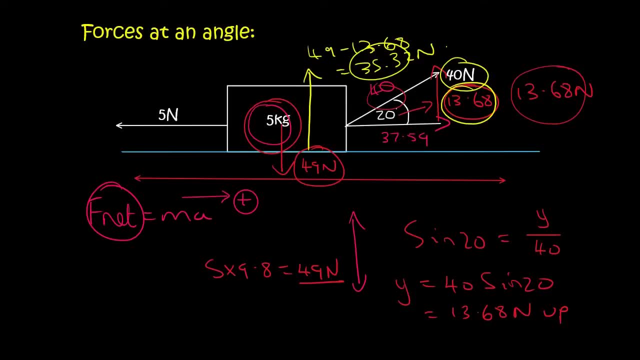 that video again, you would see that I said in this type of question the normal force is the same as gravity. If you have an object- and I'm getting far ahead of myself, I only wanted to do this in like the next lesson or two- If you have an object where there is a force that is going to 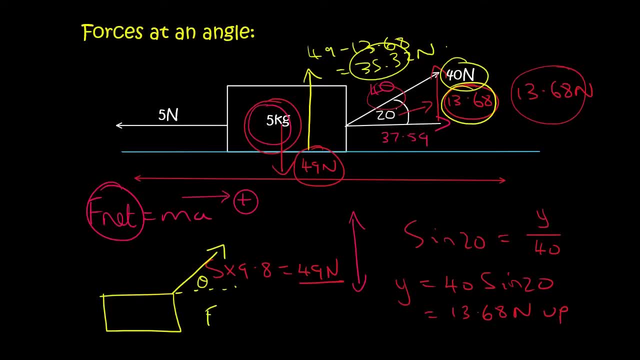 applied at an angle, then your normal force is not the same as the force of gravity. That is very important, But I will explain that in detail in future videos. So I did that just to show you that you don't have to worry about the object lifting off the ground And just to make sure that you 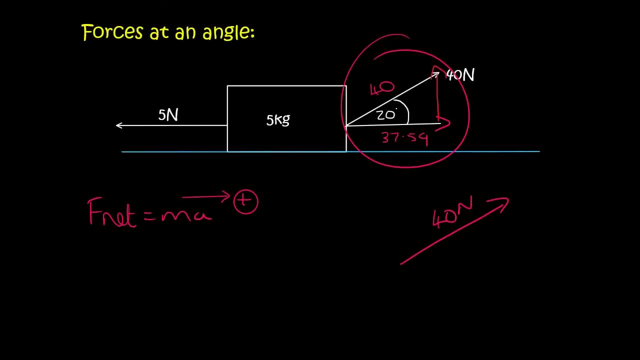 understand this part. So we have a 40 newton force, And what's more important for us is to break that up into the horizontal and then also into the vertical. sometimes in later videos you'll see that that also becomes quite important. We